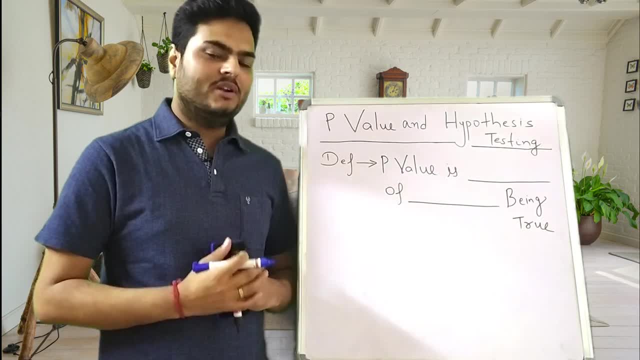 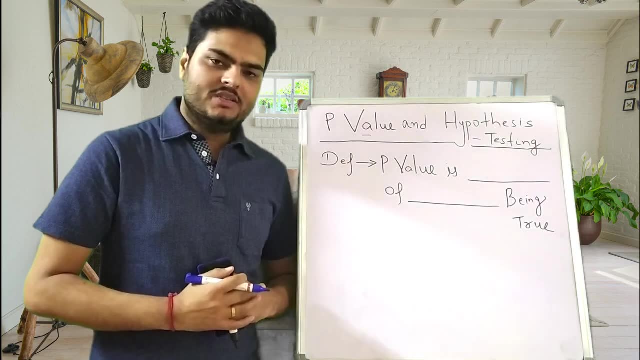 Some of the topics are unnecessarily scary in the world of data science. One of such topic is p-value and hypothesis testing. Welcome to Unfold Data Science. My name is Aman and I am a data scientist. If you watch this video till end, I am going to make 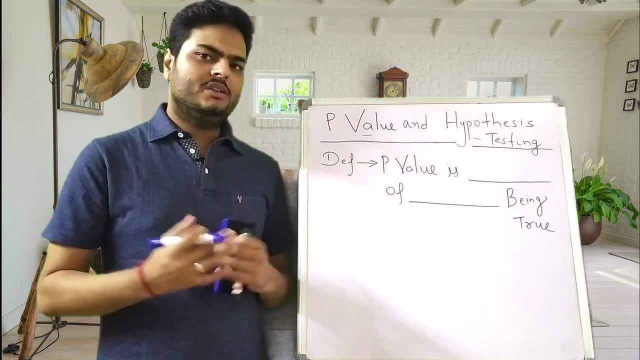 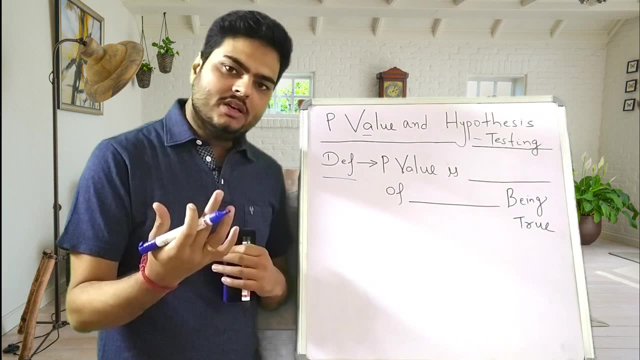 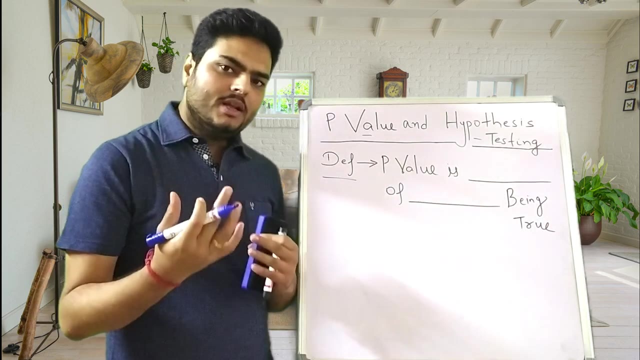 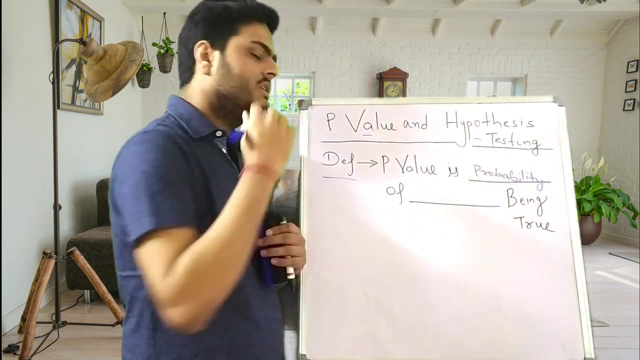 these two things extremely simple for you. Let's start the discussion. So what is p-value by definition? So I have written here the definition: p-value by definition is something of something being true. Let me fill these two blanks here. p-value is probability of null hypothesis being. 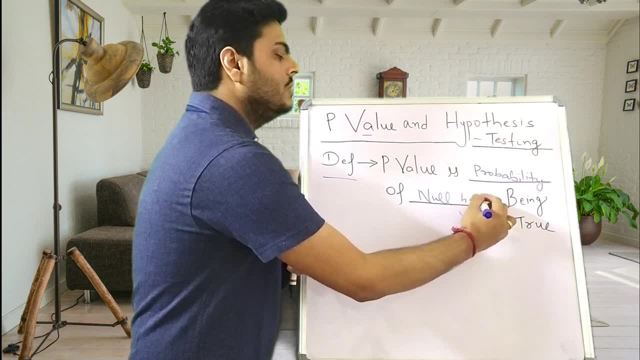 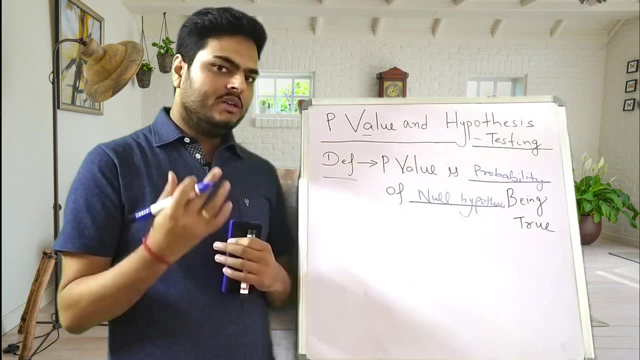 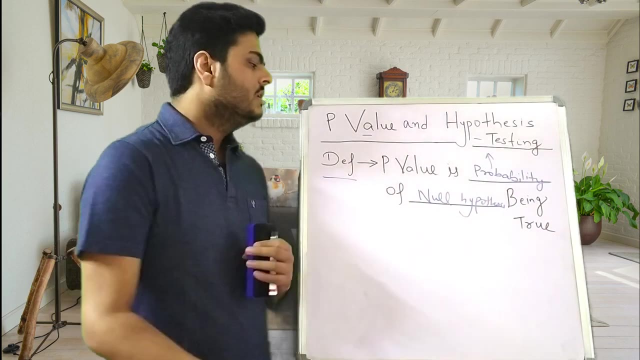 true. Now I am sure all of you must be aware of probability concept by now. If not, there is a video created by me. The link is right here. Go ahead and watch that video to understand the basics of probability. That is about probability Coming to null hypothesis. What is null hypothesis? So null? 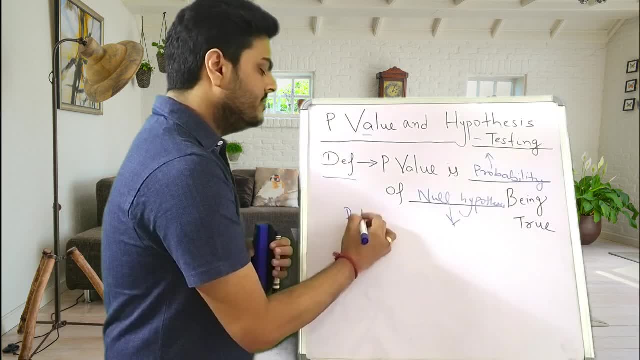 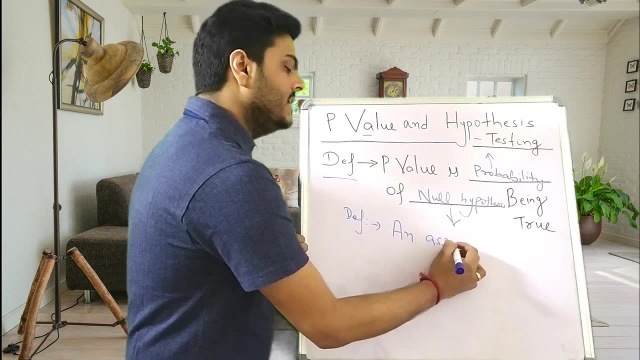 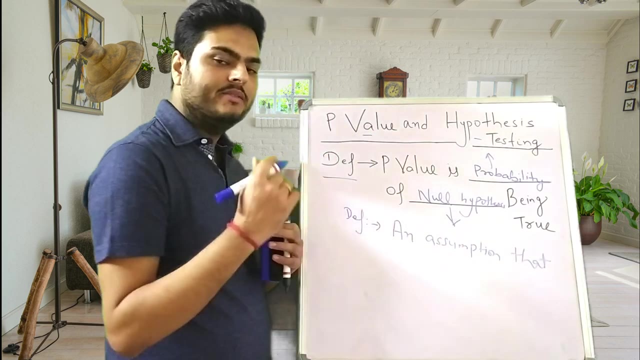 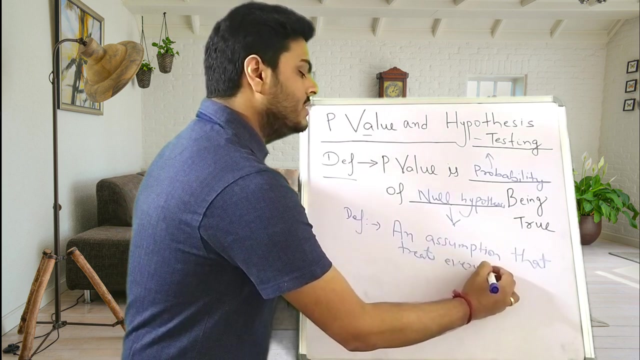 hypothesis again. we will define here. So definition of null hypothesis. I am writing here an assumption. Null hypothesis is an assumption that treats everything equal and similar. This is very important guys: An assumption that treats everything equal and similar. What will be the examples of null hypothesis? Can you think in your mind? 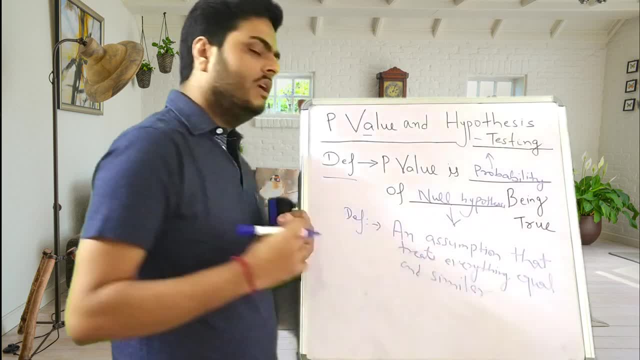 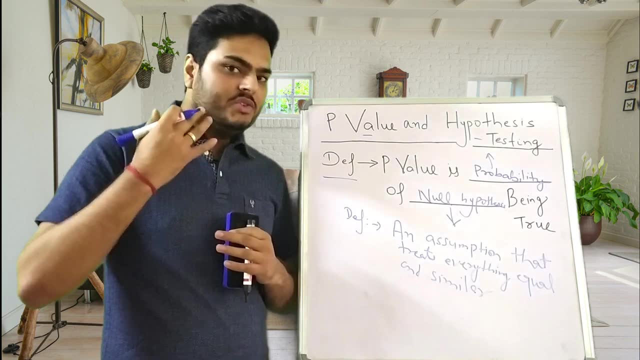 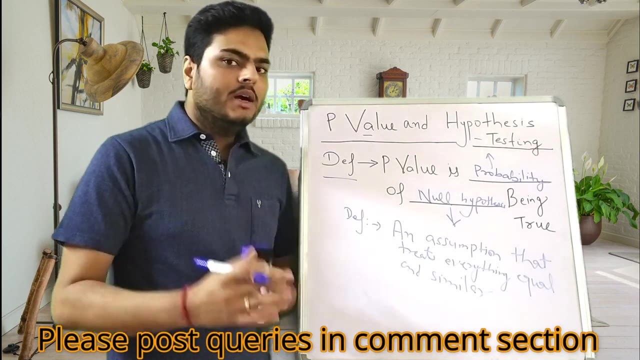 right now, For example, we are going through a lockdown due to this current pandemic situation, So a null hypothesis may assume that situation before pandemic and situation after pandemic are same. In other words, a null hypothesis will be something like GDP before pandemic. I am writing. 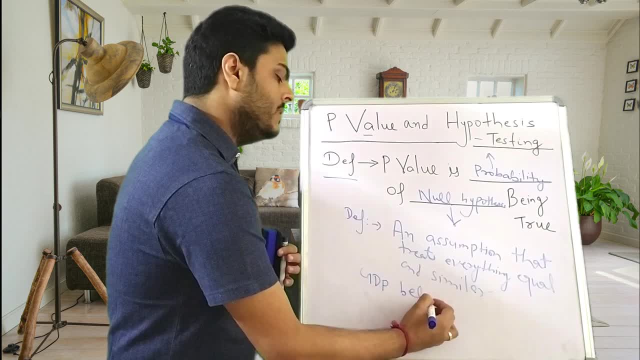 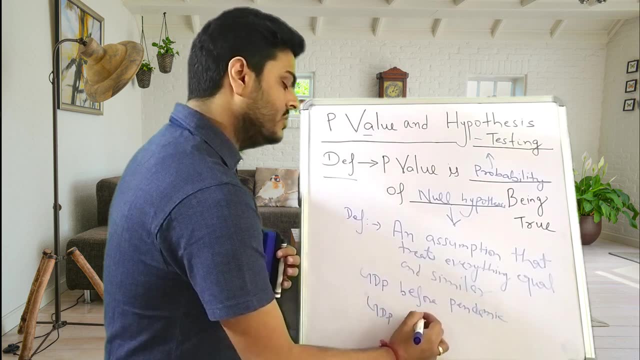 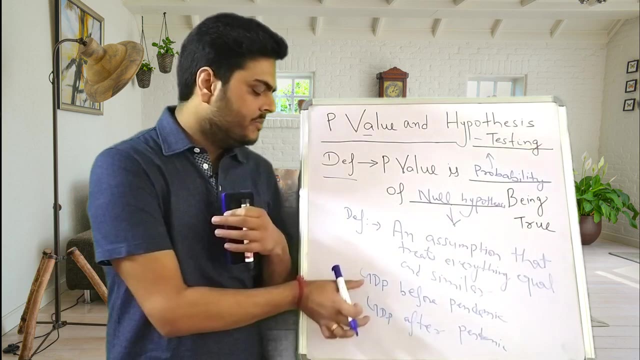 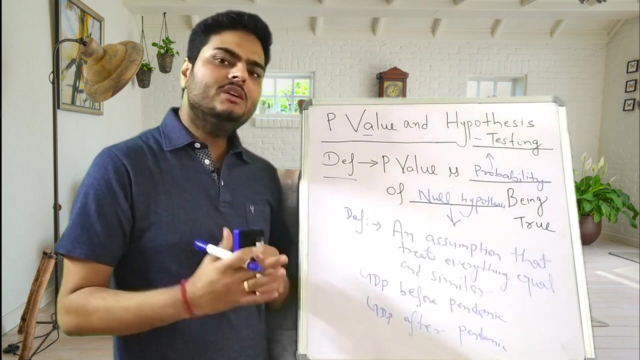 a statement here. GDP before pandemic and GDP after pandemic. I am talking about global GDP here. GDP before pandemic and GDP after pandemic are same. So this is a statement which treats the before pandemic situation similar to after pandemic situation. That is a default assumption. 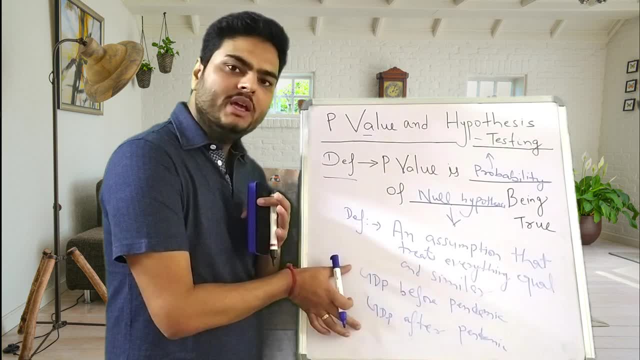 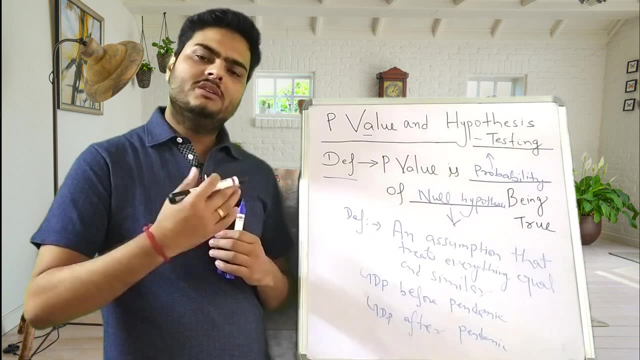 Now, logically, do you think this is a correct statement to make? GDP before pandemic and GDP after pandemic will it be same? So you must be aware that many research are going on and telling that GDP might fall by 5%. global GDP Country-wise also. it will be in. 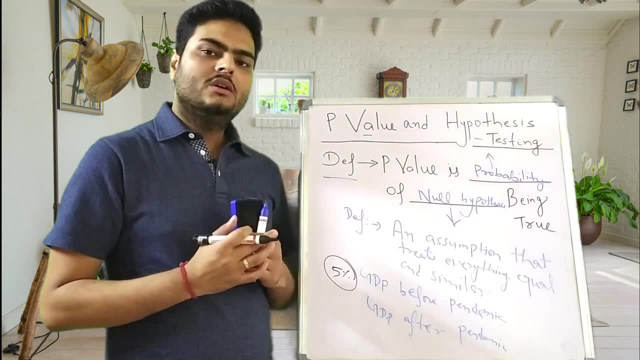 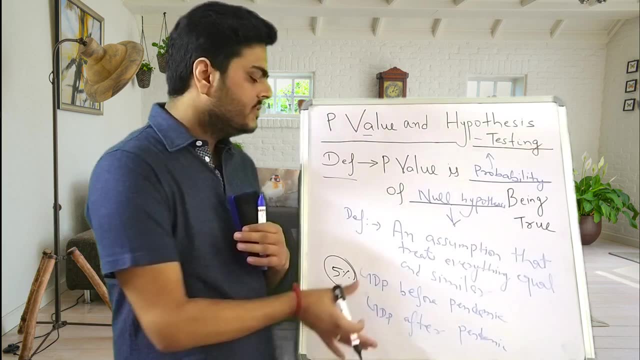 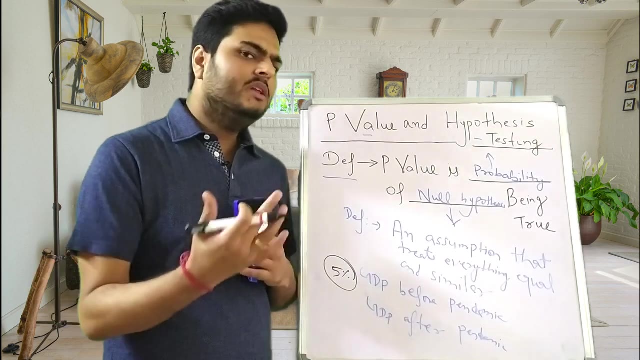 similar range as well. So this is a null hypothesis. Now, what is the use of p-value? is using the data. Using the data, you prove this hypothesis to be wrong and then you accept the alternate hypothesis. What will be the alternate hypothesis? GDP before pandemic is not equal to GDP after pandemic. 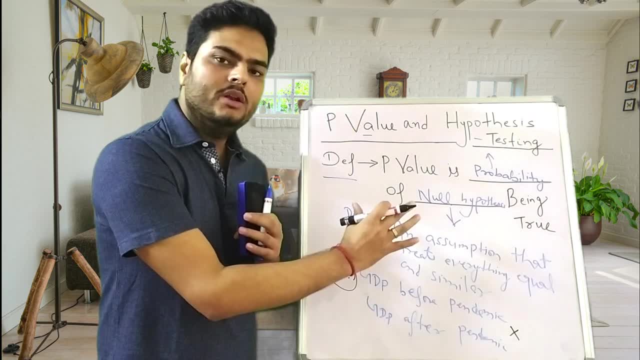 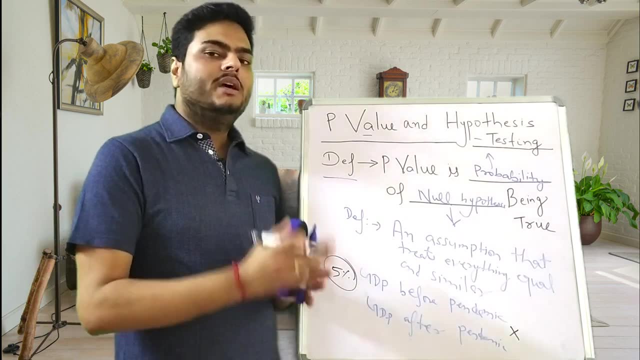 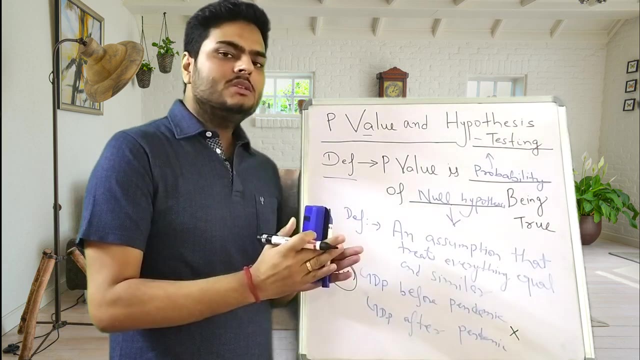 So till now, we have discussed p-value is the probability value of null hypothesis being true. And what is a null hypothesis? An assumption that considers everything to be similar and equal, All the situations to be similar and equal. Another example can be: front benchers are equally intelligent as the back benchers. This is another assumption. Means all the 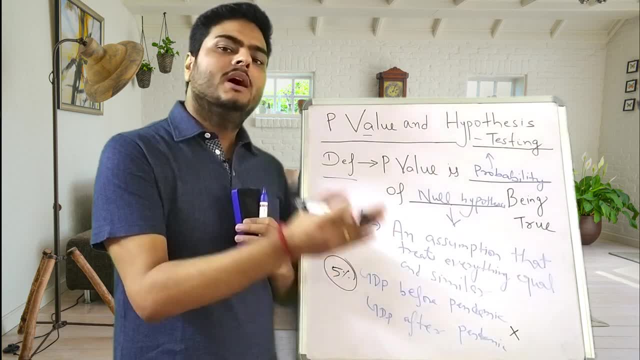 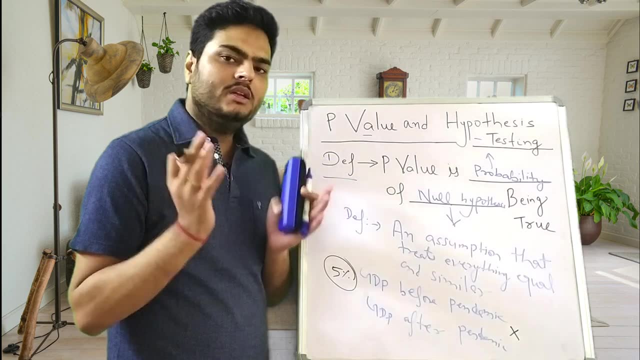 in the class are equally intelligent. Front benchers are equally intelligent as the back benchers. How can you prove this statement as wrong? You compare their marks and then you say: you know what front benchers are scoring more, hence they are more intelligent. 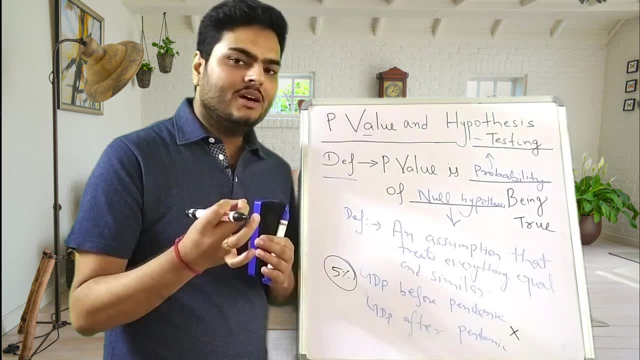 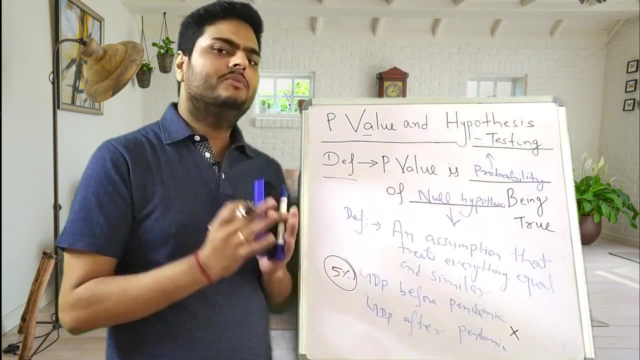 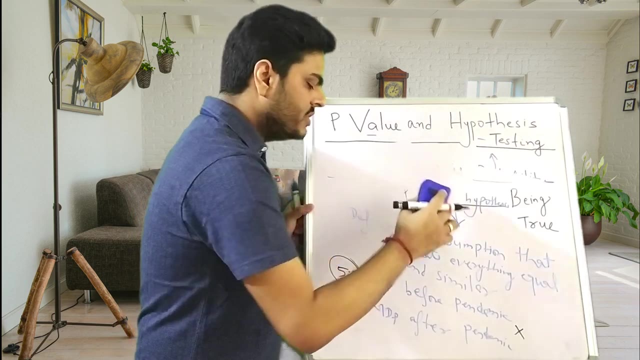 Back benchers are less intelligent. So with the data and p-value, you either accept a null hypothesis or reject a null hypothesis. This is by definition. Now let us see what process do we follow when we go and do the hypothesis testing? This process that we discussed now is known as 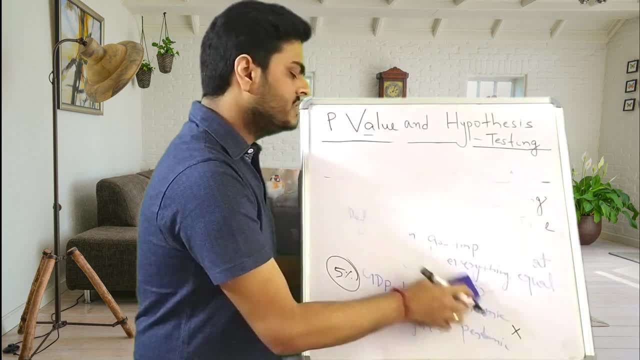 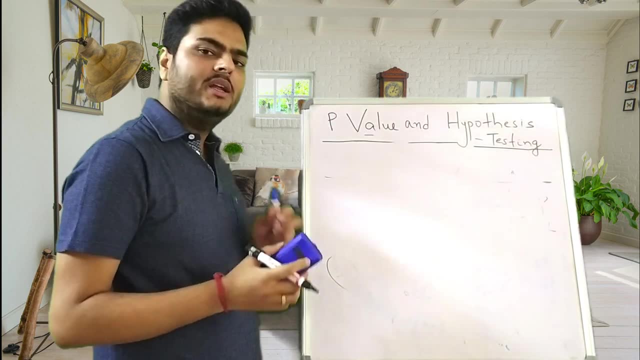 hypothesis testing. Okay, So what is hypothesis testing? The process of accepting or rejecting null hypothesis. How do you do hypothesis testing practically? So, in our GDP example, if you have to prove whether null hypothesis is right or wrong, what you will do? 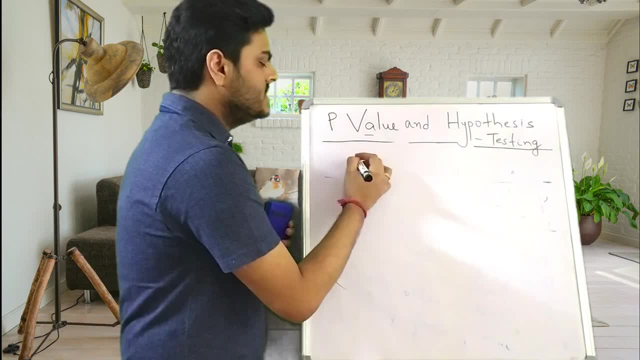 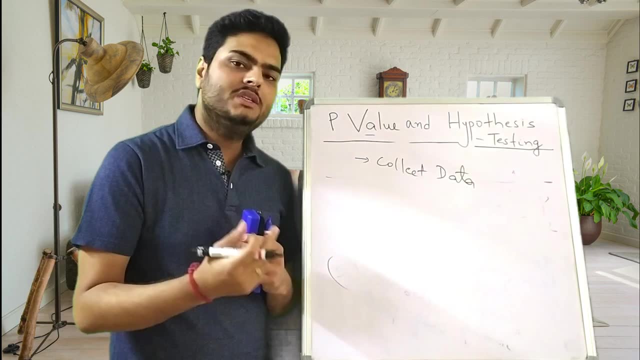 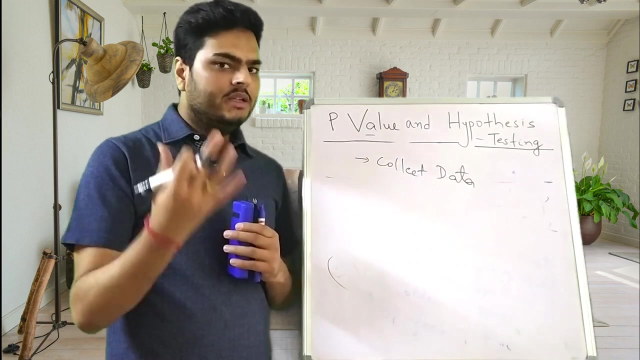 you will go and collect the data, right. So very first step will be: collect data. Okay, What data you will need for to prove that GDP before pandemic is different from GDP after pandemic? You will take the GDP of different countries in the world, right, And then that. 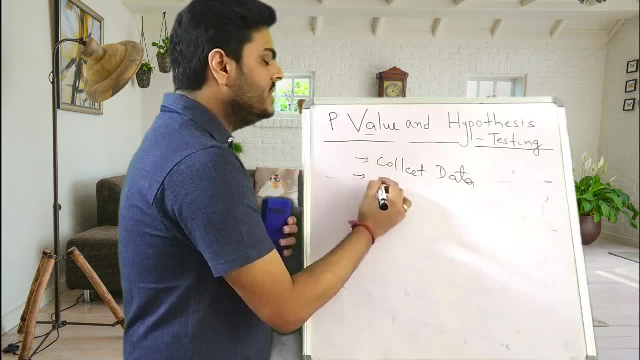 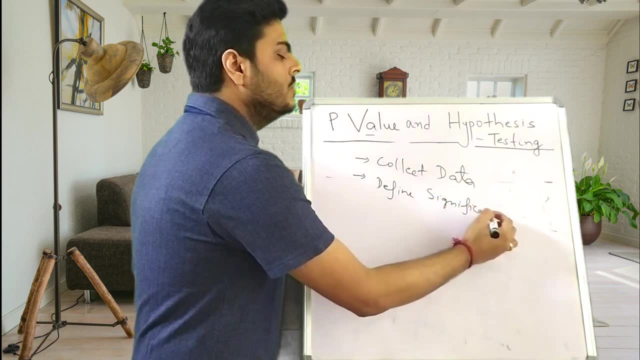 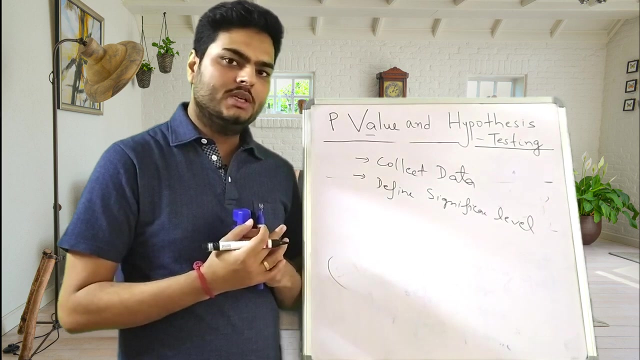 becomes your data. Next is your significance level that you have to define, Define significance or significance level. Now, what is the significance level? So I'm sure if you are into data science for some time or you have been watching some tutorials, you know there is an. 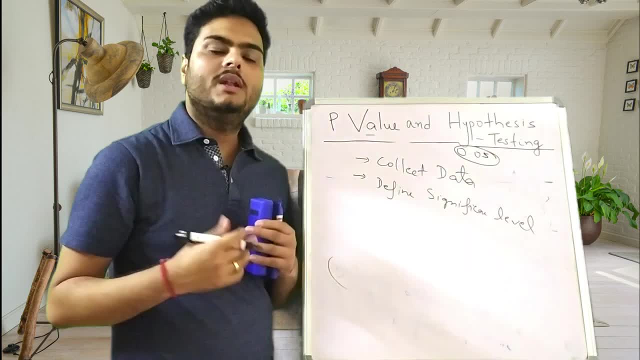 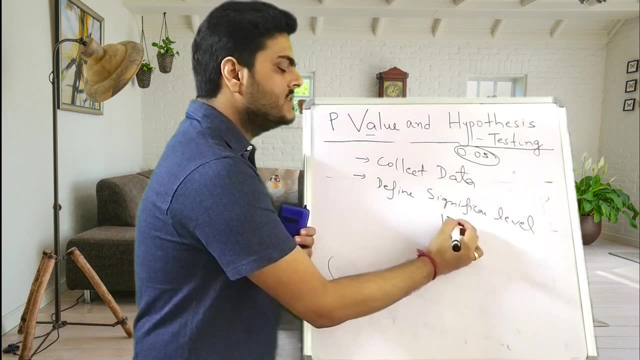 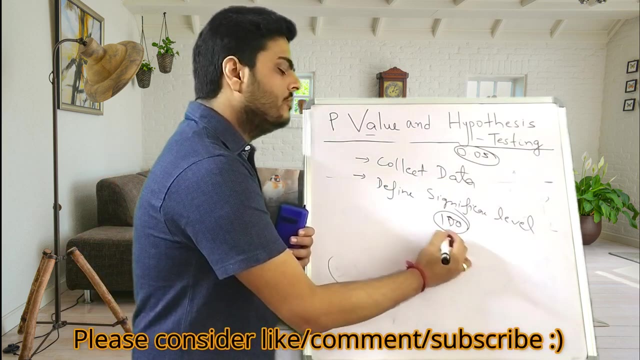 early definition of 0.05 for P value, the significance level. The meaning of this 0.05 is if I take data of 100 countries at random. if I take data of 100 countries at random, then 5% or 5 countries, the GDPs will be same, which means for 5%. 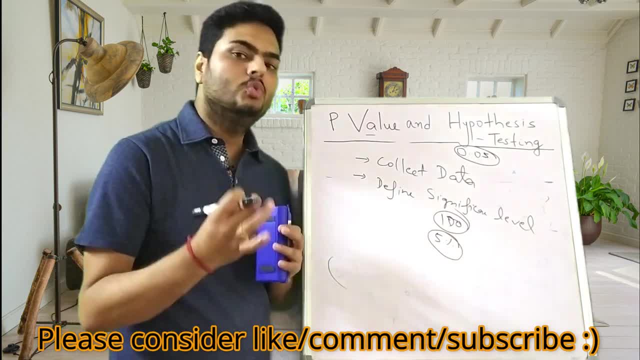 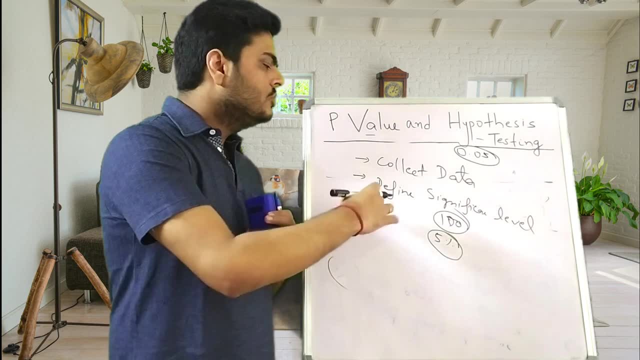 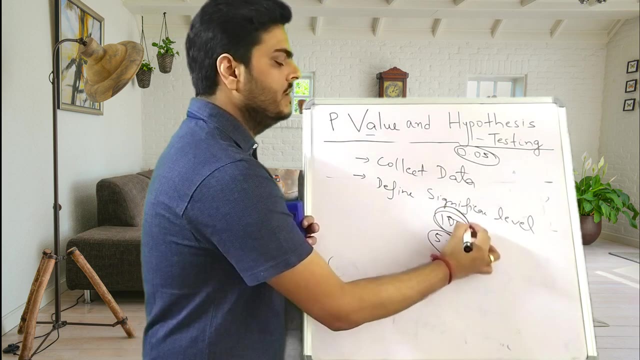 of the cases is the null hypothesis will hold true. That is the significance level that we fix with p value. okay, to give you with with another, to make you understand with another example. you can say like this: if you take 100 country gdp- gdp before pandemic, gdp after pandemic- 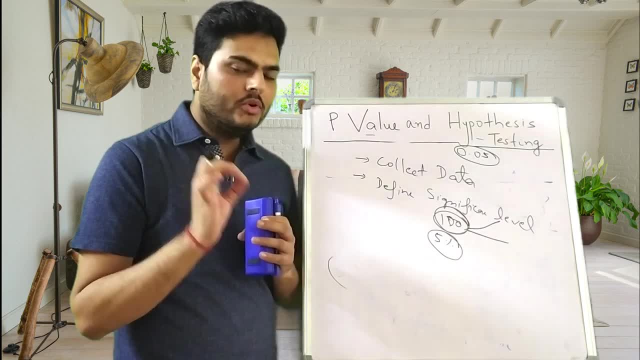 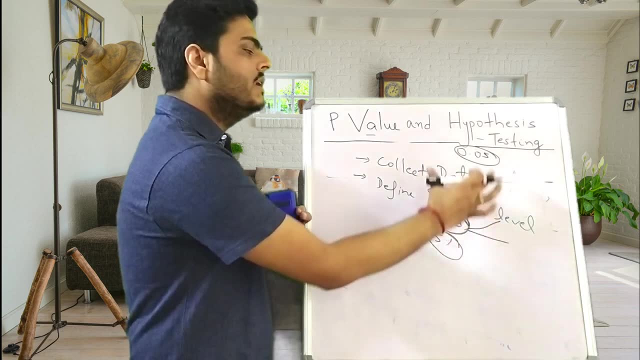 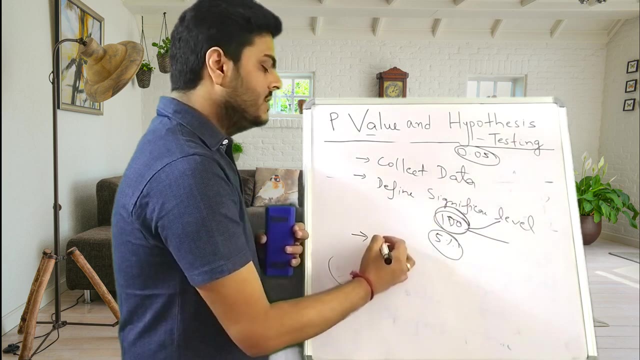 then null hypothesis will be true. for how many cases? five cases. so that is, by definition, how null hypothesis can be used and how significance level can be used. what next? if you have a significance level, if you have the data, then you can either accept or reject null hypothesis. 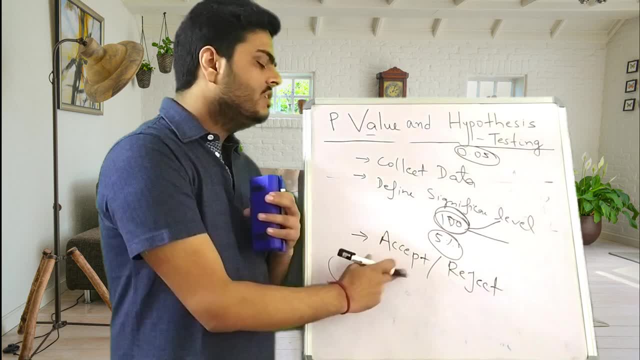 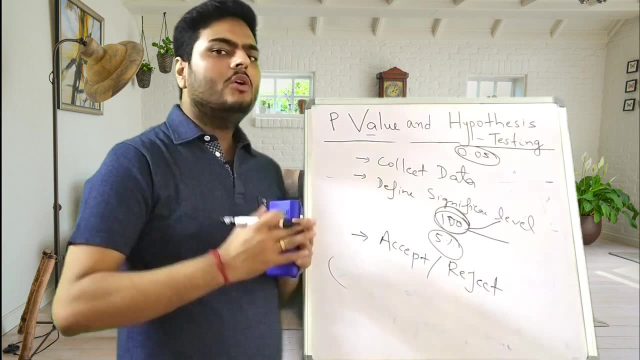 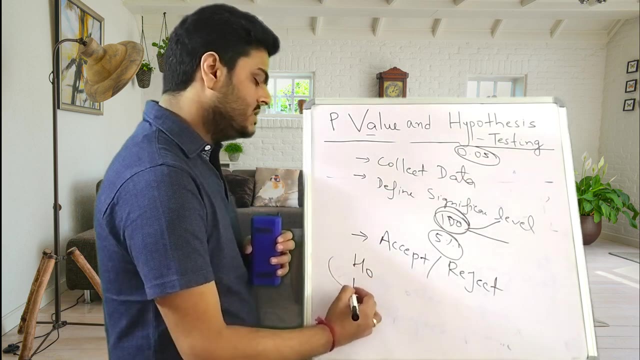 either accept or reject null hypothesis. the meaning of accepting null hypothesis is you accept what has been said as null hypothesis. the meaning of rejecting is you accept the alternate hypothesis. so what will be the alternate and null hypothesis? by definition, they are written as h naught and h a, so h naught stands for 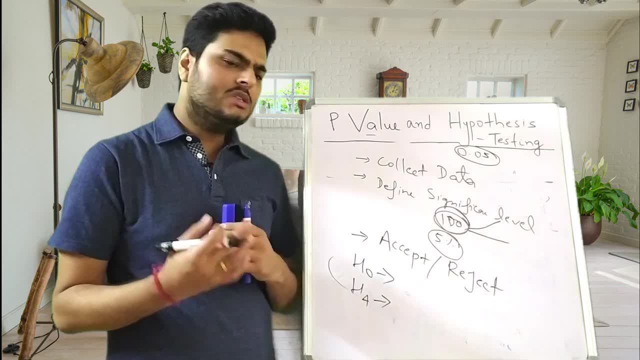 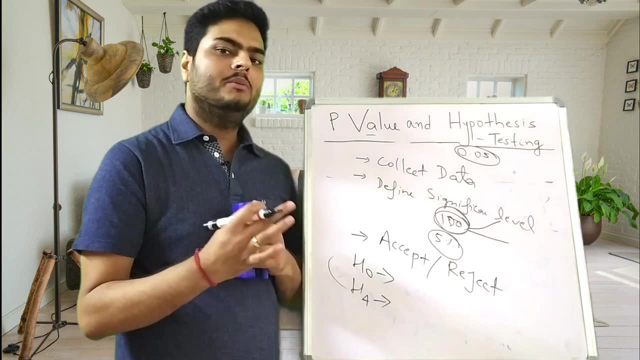 null hypothesis and h a stands for alternate hypothesis and null hypothesis. in our case, h naught will be gdp is same before pandemic and after pandemic. h a will be gdp is not same before pandemic and after pandemic. that is how, at high level, p value and 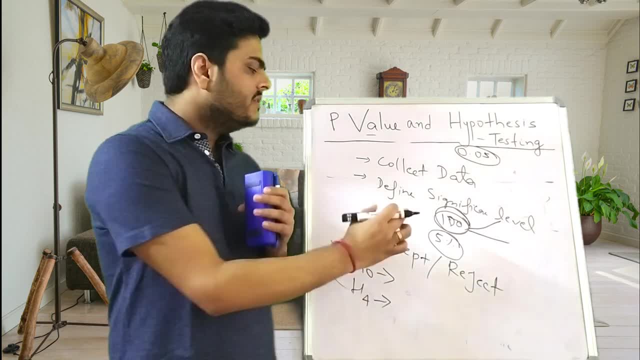 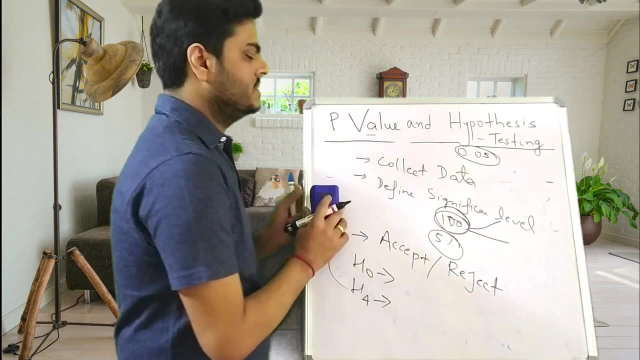 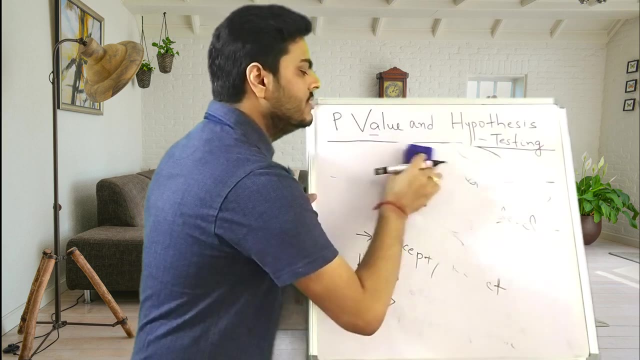 hypothesis testing works. now there is one step in between. once you have defined the significance level, then you have to do certain test to get this p value. so what are those tests? okay, so you need to do certain tests to get this p value- statistical test you would have heard of. I am just going to write down here some of 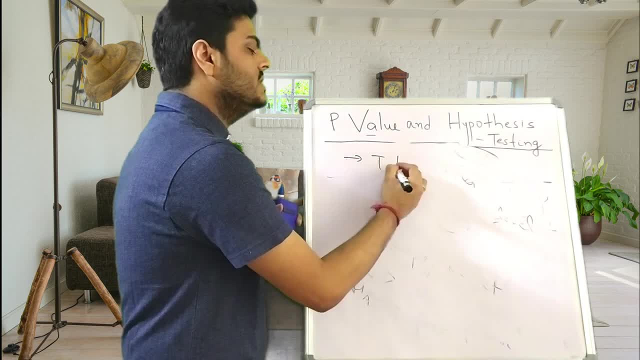 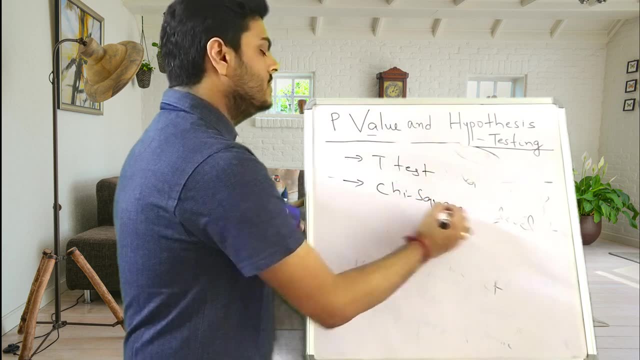 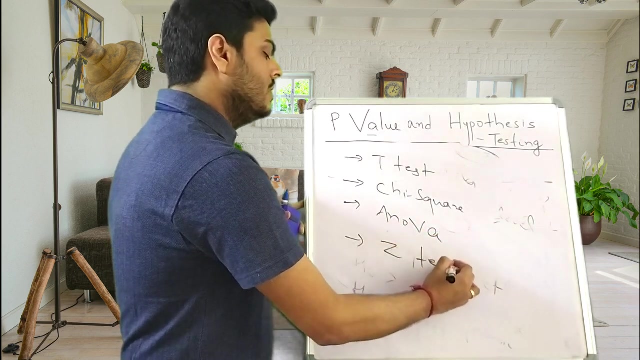 the test. So, if you have heard of something known as t-test, if you have heard of something known as chi-square test, if you have heard of something known as ANOVA, if you have heard of something known as z-test, all these are different, different test that is done on the 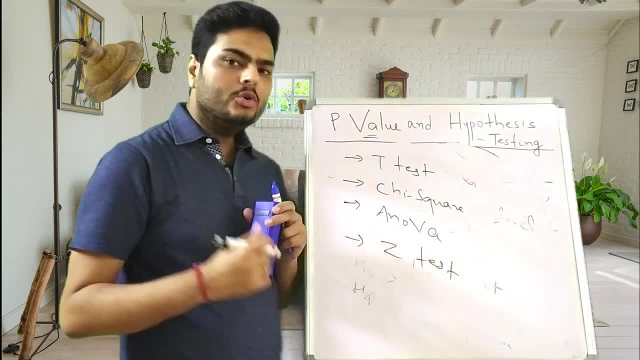 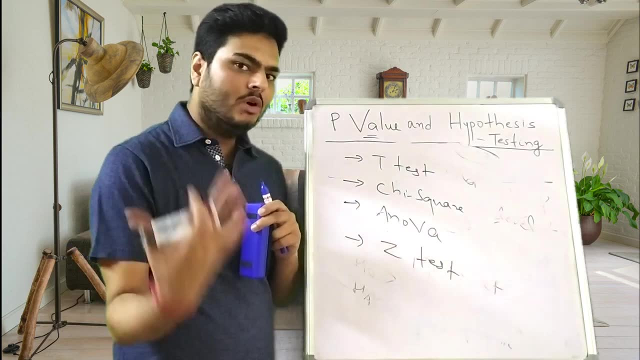 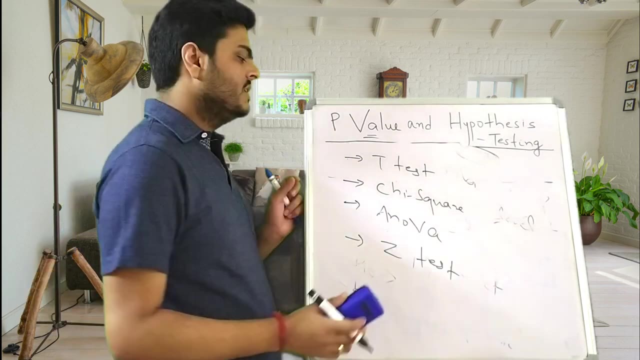 data to obtain the p-value. Now how do we interpret p-value Using the significance level? Now we have the data, we have the test and we have the p-value output. Then we can select or reject the null hypothesis. So what significance level is chosen normally? 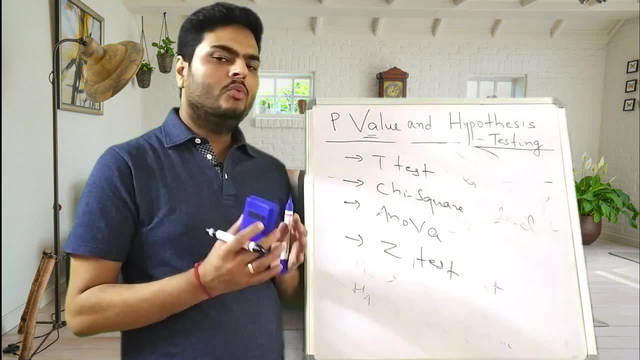 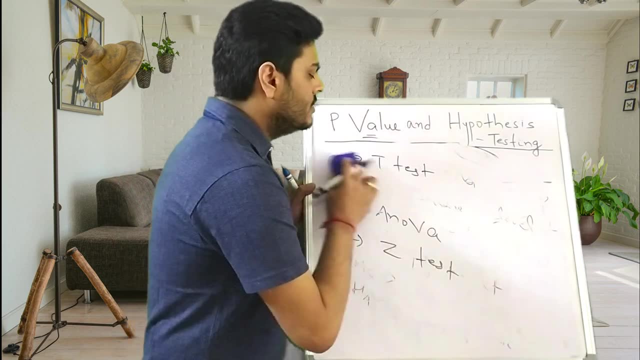 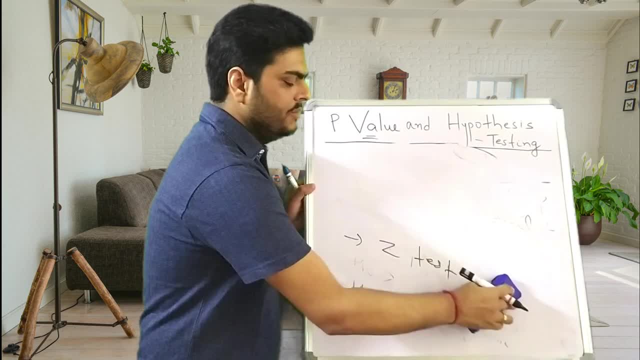 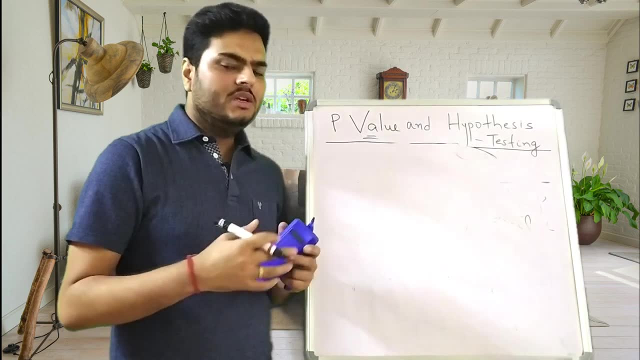 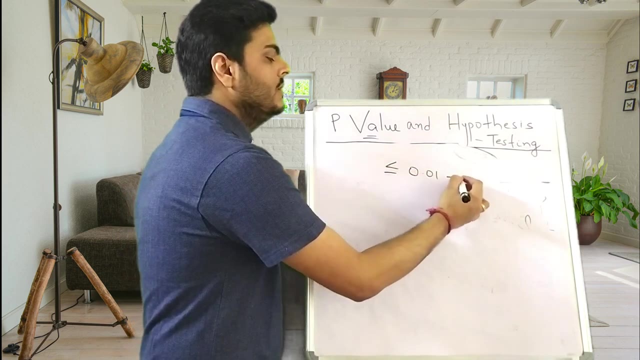 significance level tells you what is the strength of your null hypothesis or what is the with what confidence you can reject or accept the null hypothesis. So in industry there is a common practice where, if your p-value is less than 0.01,, if your p-value is less than 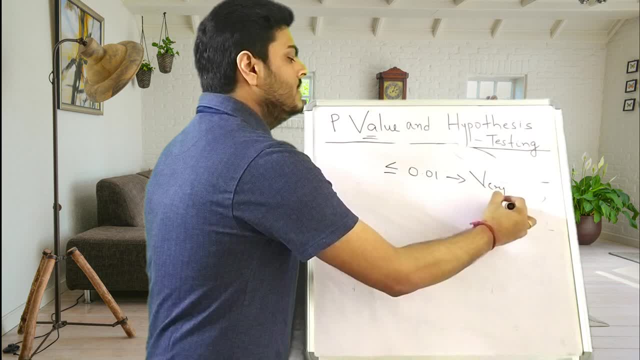 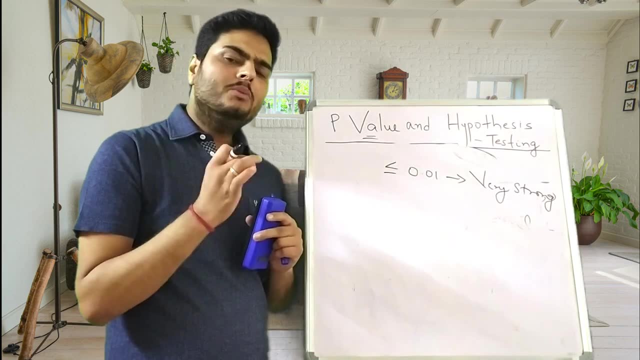 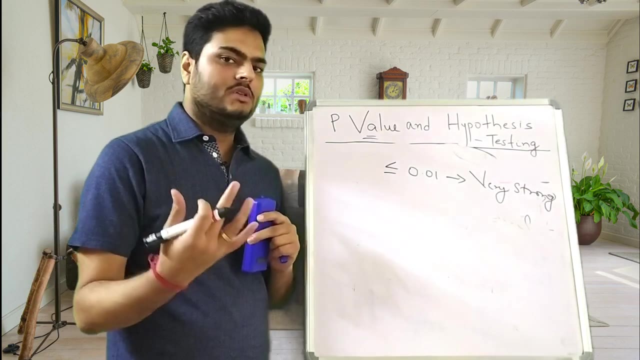 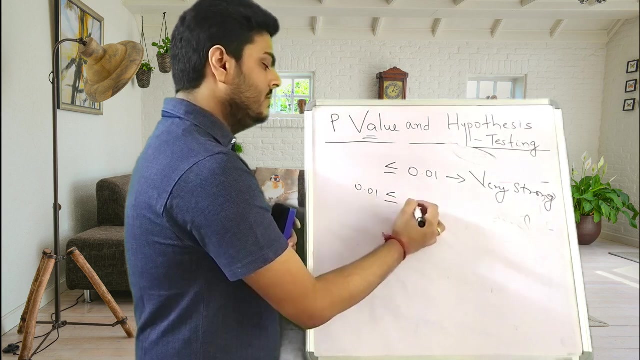 0.01, then you have a very strong case against null hypothesis. The meaning of this is: only in 1% of the cases your null hypothesis will hold true. In 99% of the cases, your null hypothesis will be false. If your range is between 0.01 to p-value, 0.01 to 0.05, then we say that 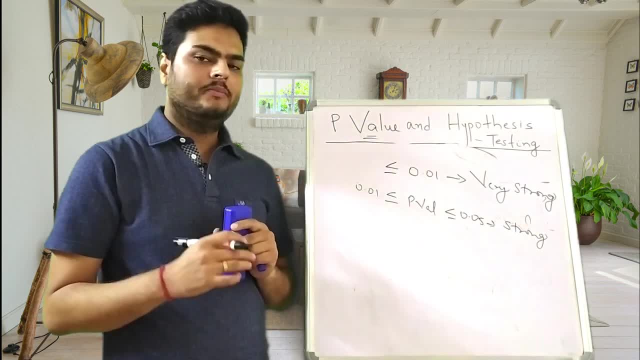 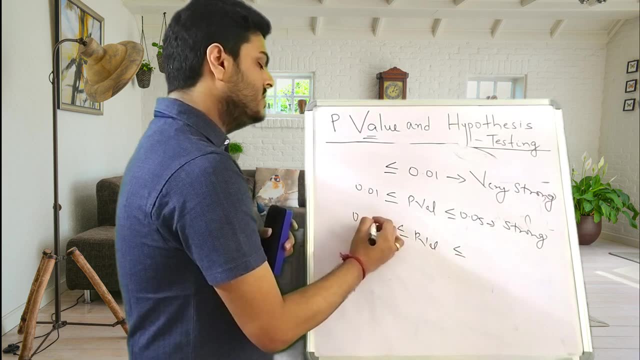 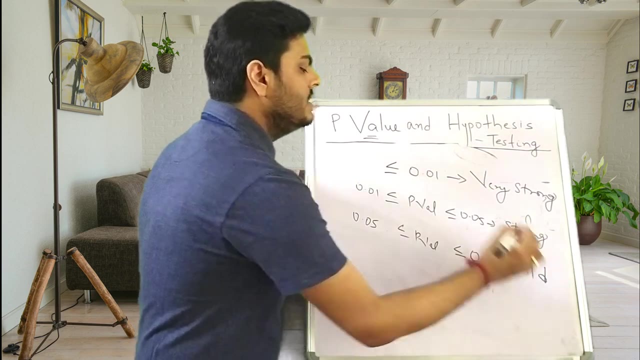 it is a strong evidence against null hypothesis. If this range expands further, for example, if your p-value is in the range of 0.01 to 0.05, then it is a strong evidence against null hypothesis. If your p-value is in the range of 0.05 to 0.01, then you can say mild evidence against null. 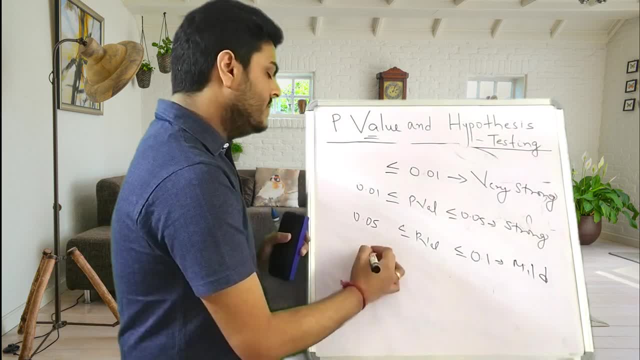 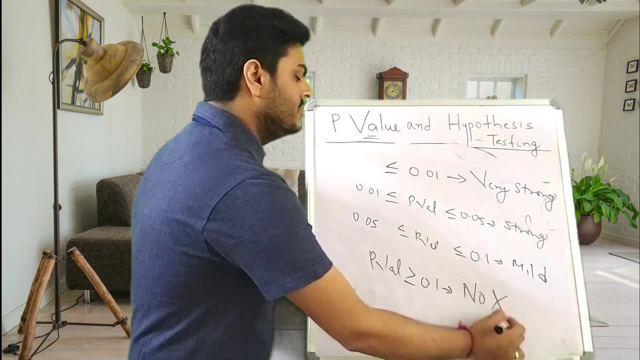 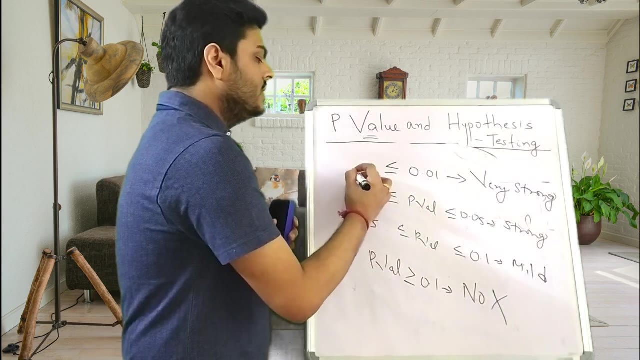 hypothesis And if your p-value becomes more than 10% or more than 0.1, then you can say no evidence against null hypothesis and you accept the null hypothesis in this case. So what you would have seen in general. you know internet blogs everywhere- that this is the range that